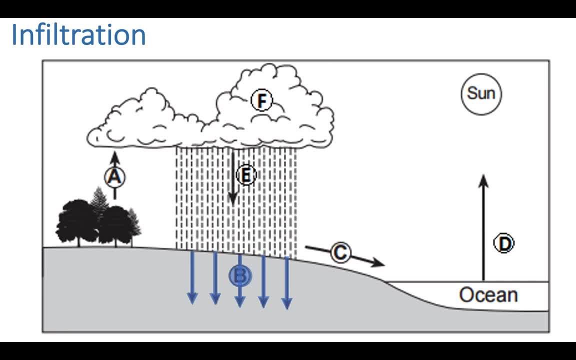 a few options. The first option is infiltration, where water goes into the ground or that water can become what we call runoff, which means that water stays on the surface of the Earth. The lesson for today is mainly the difference between infiltration and runoff, and the factors that determine whether 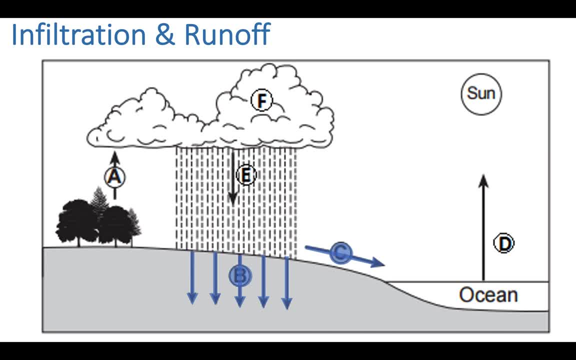 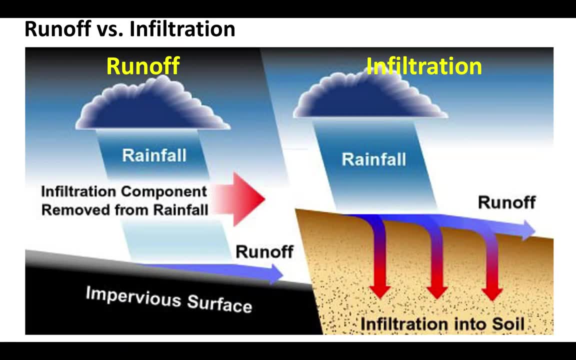 water goes into the ground as infiltration or stays on the surface as runoff. So, looking at the water cycle a little more closely again, runoff is when water goes into the ground and the factors that prevent the water from going into the ground so it stays on the 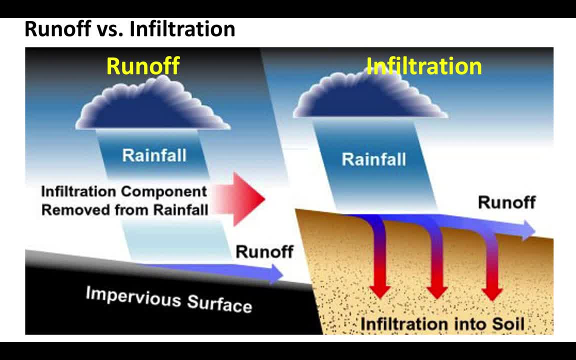 surface as lakes, rivers, oceans and even puddles after a rainstorm. Infiltration, on the other hand, means the water is going into the ground, So after a while you don't even know that the water was there anymore, because it's gone and was stored underneath the ground. 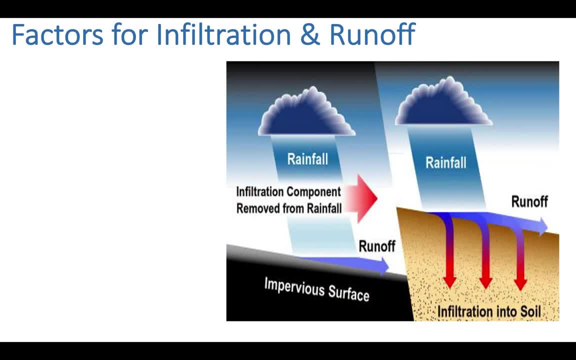 as something called ground water. Now, there's different factors that affect infiltration and runoff. One of them is the factors that can influence whether water is going to infiltrate or become surface runoff. The first is the slope of the land. The second is the size of the soil particles that make 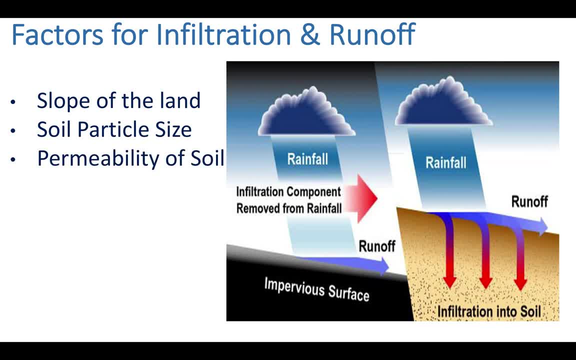 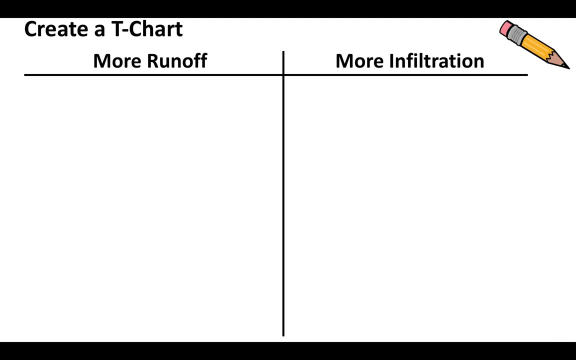 up the ground. The next is the permeability of the soil, the saturation of your soil and, finally, whether your ground is made up of vegetation. Throughout this lesson, you're going to see this symbol in your notes, which has a T-chart and a pencil symbol, which means 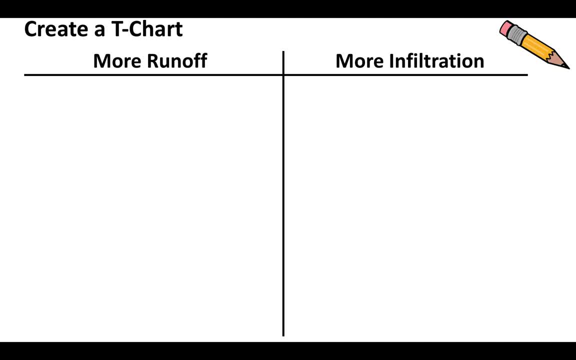 you should be writing this in your notebook. We're going to make a T-chart so we can put the factors that will lead to either more runoff or more infiltration. So this is going to be an ongoing chart that we fill in as we go through the notes. 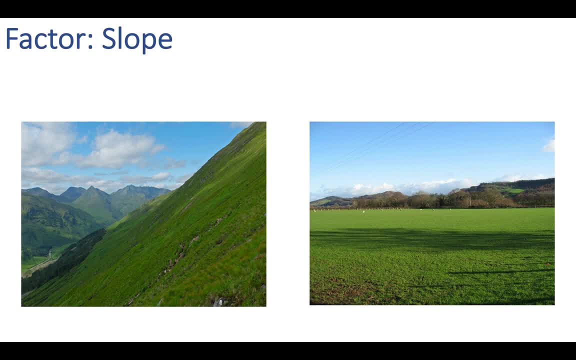 So we're going to start with the first factor, which is the slope of the land. On the left side of the screen, you can see that that picture is showing a steep slope, while on the right side, that picture is showing a flat slope. When rain hits the surface with a steep 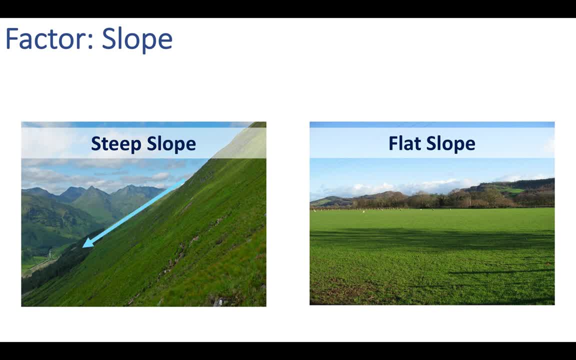 slope, that rain hits the ground and the ground gets drenched heavy. Remember, the USDM is going to just run off of the slope. It's not going to be able to go into the ground. It's going to hit the ground and then keep sliding off. Think of a really awesome steep water slide. 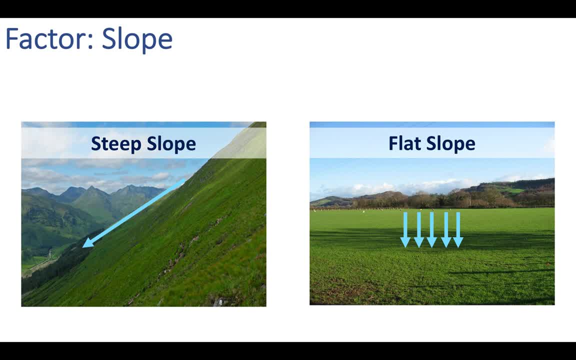 On the other hand, when rainwater hits a flat slope, there's going to be enough time for that water to hit the ground and then settle in and infiltrate the surface. So when you have a steep slope, you have more runoff. When you have a flat slope, you're going to have more infiltration. 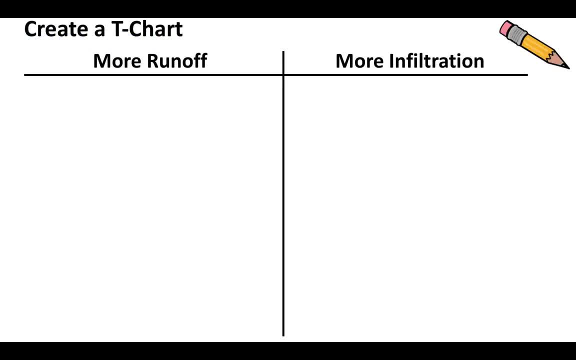 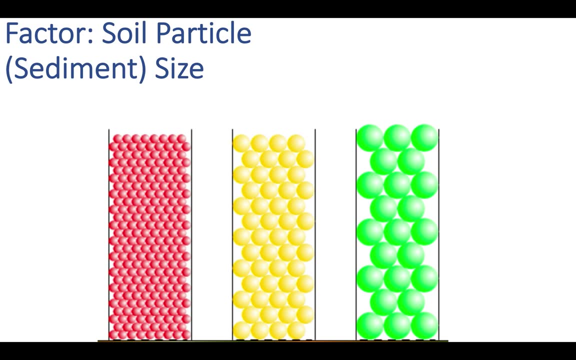 So make sure you go back to your t-charts and you add: there's more runoff when you have a steeper slope, more infiltration when you have a flatter slope. The next factor is going to be soil particle or sediment size. So here we have three different sized sediments: small, medium and large. And if 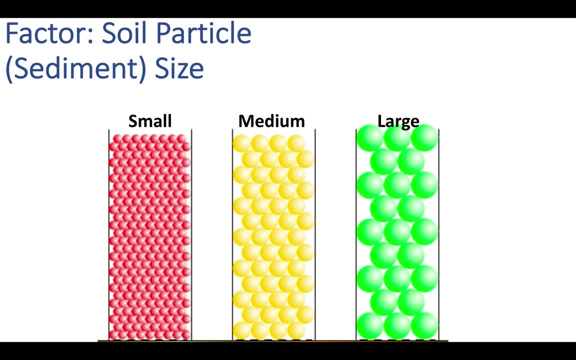 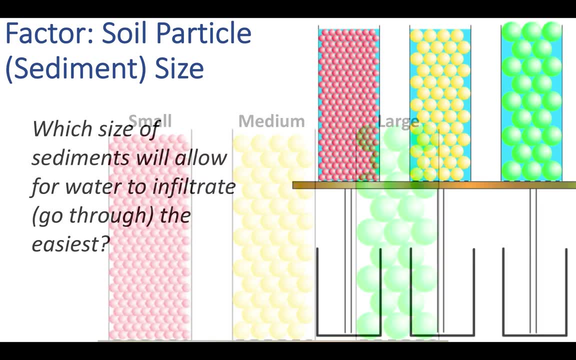 water were to hit the top of these three columns of different sized sediments, the size is going to increase. So you're going to have more runoff. when you have a steeper slope, more infiltration and more impact Which one allows water to go through. So our question becomes: which size? 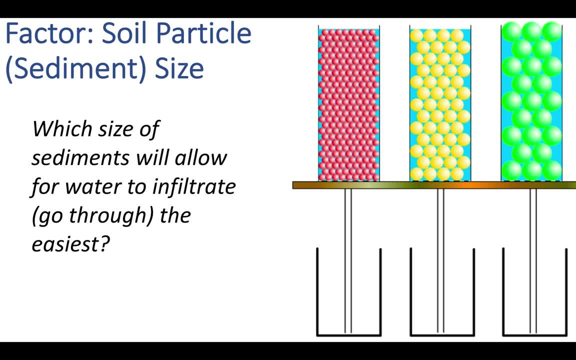 sediment will allow water to infiltrate, which means go through the easiest. On the right side of the screen it's going to be an animation, and you can see behind the sediments that they're each filled with blue water, So each of the containers are filled to the top with water When I press the. 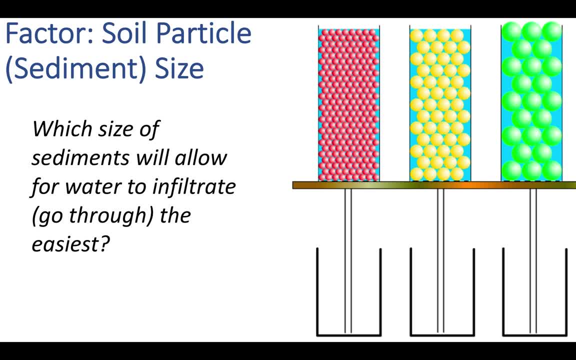 play button, we're going to see which container allows the water to go through the easiest. That means you're going to have the most infiltration. So if you're going to have the most infiltration, you're going to have the most infiltration. So after viewing that animation, you can see that the 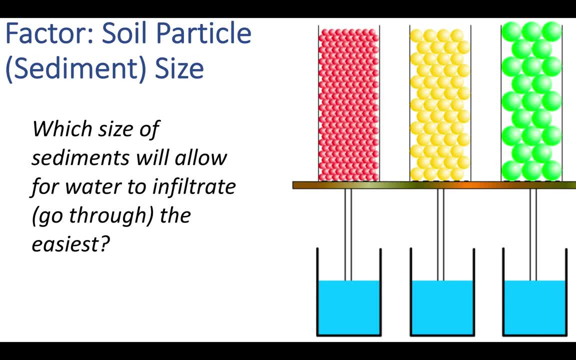 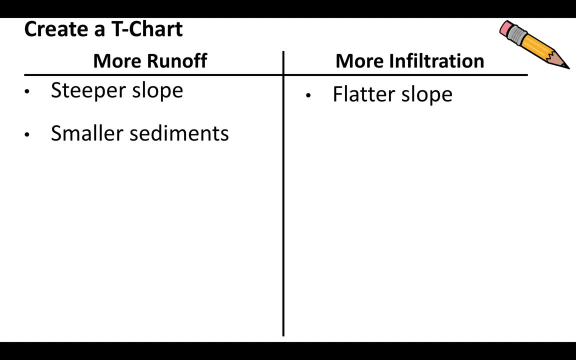 large green sediments allow for the water to go through faster. The water was able to infiltrate more, So larger sediments allow for the most infiltration. So if you go back to our T chart, you'll have more runoff. where the soil is made up of small sediments, It's going to be really 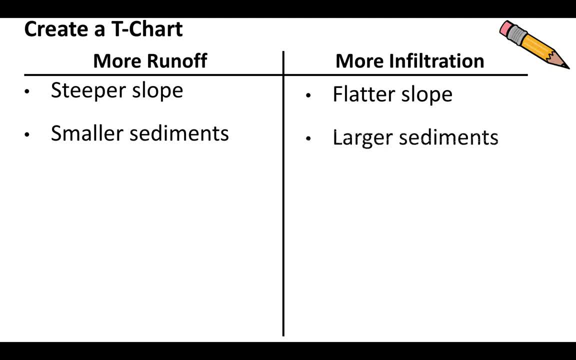 hard for water to get through smaller sediments. When you have larger sediments, you're going to have larger sediments. The water will infiltrate a lot greater. So a ground consisting of large sediments, more infiltration. Another factor is permeability of soil, which means the ability of 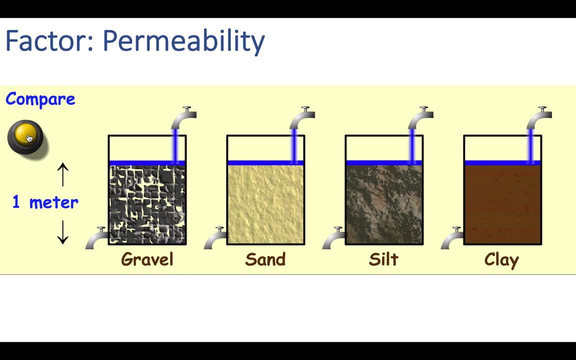 water to pass through. So it's very similar to the definition for infiltration, which also means water to pass through the surface. In this animation that we're about to play, we have different types of sediments. We have gravel, sand, silt and clay, which goes in size order. 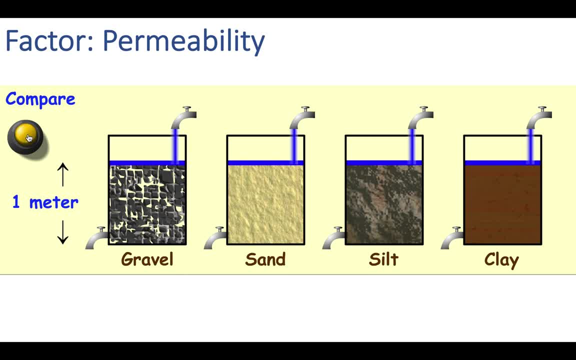 Gravel is the largest sediment. Clay is the smallest. As we fill up these containers with water, take a look at what happens. The gravel allows for the most infiltration, which makes sense because the sediments are larger. but also that relates to permeability, the ability to pass through. 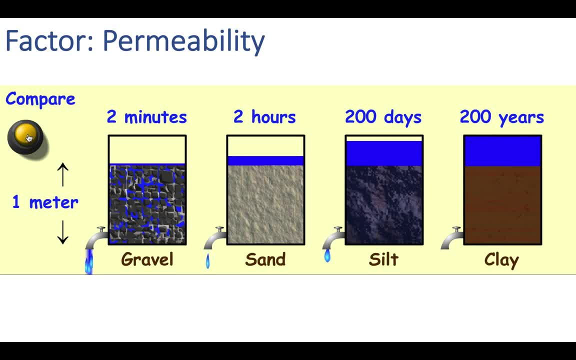 Water can pass through one meter of gravel in about two minutes. It takes two hours for water to pass through one meter of sand, 200 days for water to pass through one meter of silt and 200 years for that water to pass through the clay, the smallest sized sediment. 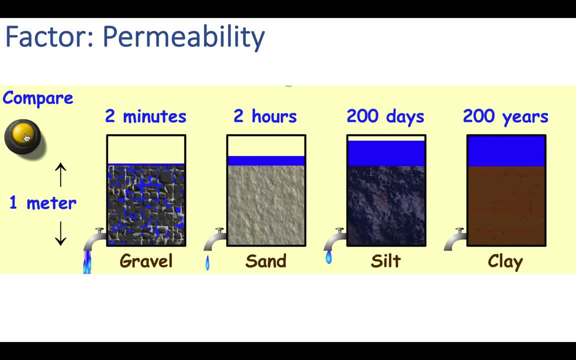 So, in short, when we have the gravel, the largest sediments, very similar to more infiltration, it's going to be the most permeable. Water can infiltrate the gravel the easiest, While on the other hand, the least permeable, we can call that as impermeable. the water cannot. 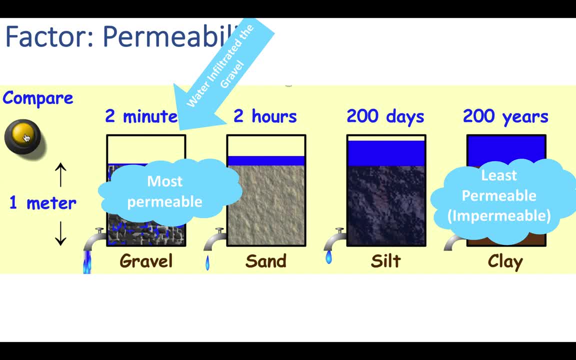 pass through that clay. It's actually still sitting on top of the surface in that animation, So that's going to mean the water is going to stay runoff. When water hits a clay surface, it's very difficult for that water to infiltrate the ground. It's going to stay on the surface. 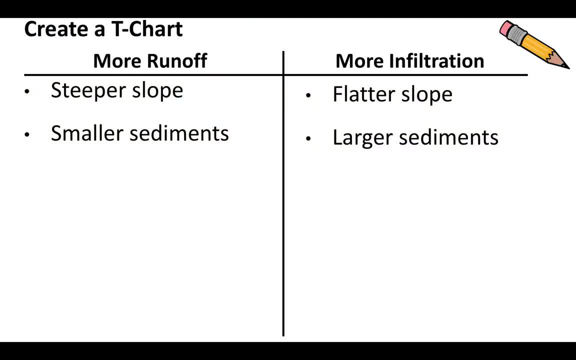 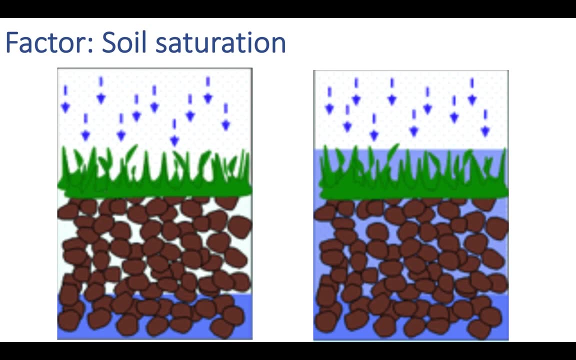 which is what we call runoff. So we're going to add that to our t charts. Impermeable soil will lead to more runoff. Where you have permeable soil, which means the water can pass through, will lead to more infiltration. Another factor that can influence infiltration and runoff is 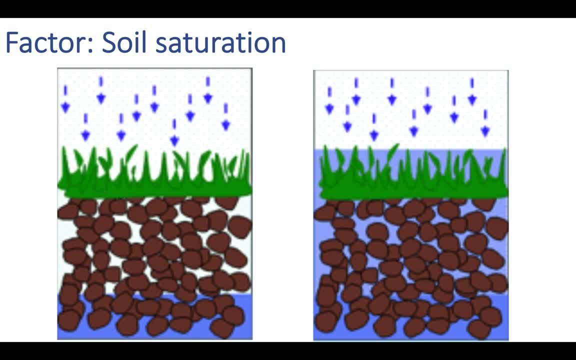 soil saturation. I want you to think of the word saturation as to be filled with. If you are saturated, you are filled with water. Think of a dry paper towel versus a wet paper towel. A wet paper towel is saturated with water. It's already filled with water. 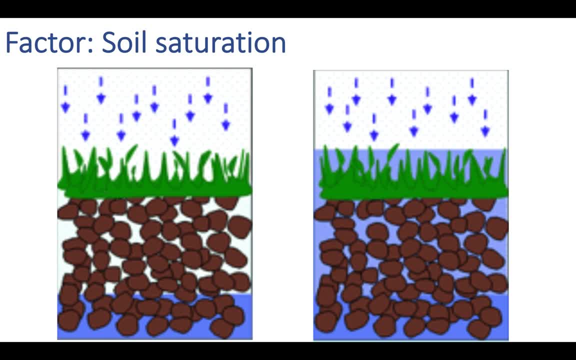 while a dry paper towel is unsaturated. It's not filled with water. So here we have, on the left side, unsaturated soil. That blue water is not completely filled within that soil. It's unsaturated. There's room for water here. On the other side picture, the soil is completely. 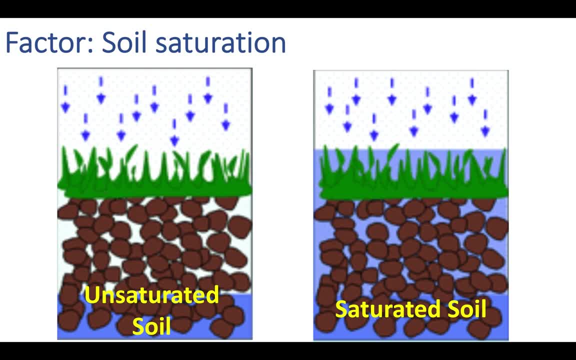 filled with water, The water reaches the surface where the grass is. That soil is completely saturated. So you're going to have more infiltration with unsaturated soil because there's room for water to fill up. On the other hand, when you're completely saturated with soil, 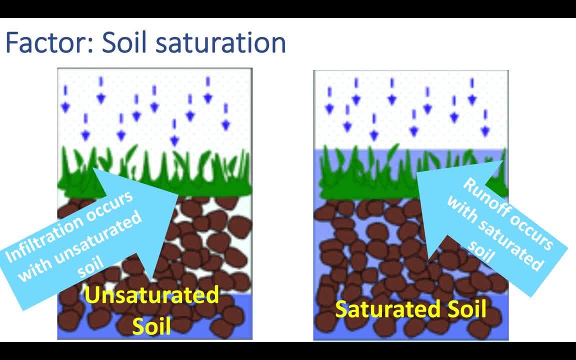 and saturated with water in your soil, and the water is all the way up to the surface already. that's when runoff starts to happen, because there's nowhere else for the water to go but to stay on the surface. There's no room for that water to go into the soil, So it becomes. 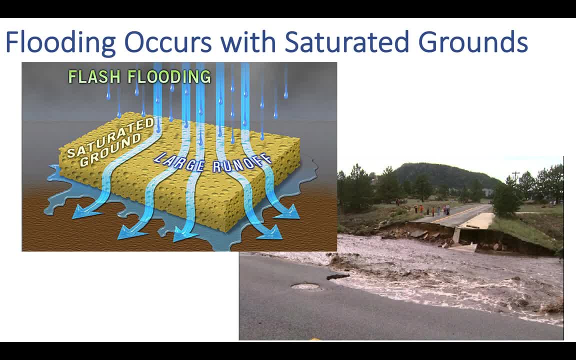 runoff on the surface of the earth Anytime you have flooding events. that's when you have your ground is completely saturated. There's nowhere else for the water to go, so it must stay on the surface of the earth. So you have a large amount of runoff during major flooding events. So make 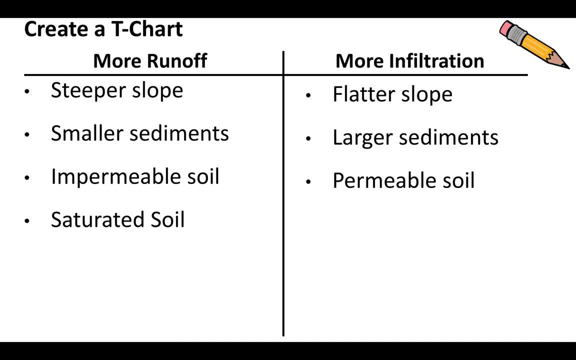 sure you add to your t chart. saturated soil is going to lead to more runoff. When you have unsaturated soil, you have room for the water. So as the water is hitting the ground, there's room for the ground to soak up that water, with unsaturated soil leading to more infiltration. 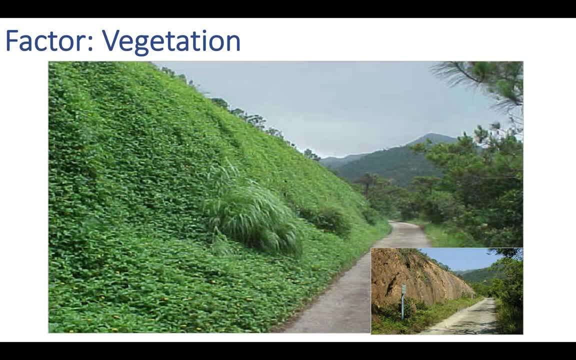 Now, finally, our last factor is vegetation. Vegetation- think of the word vegetable, Think of all the green vegetables that you need to eat to stay healthy. When you have a lot of vegetation, that means the land is covered with vegetation, So you need to have a lot of vegetation. You need 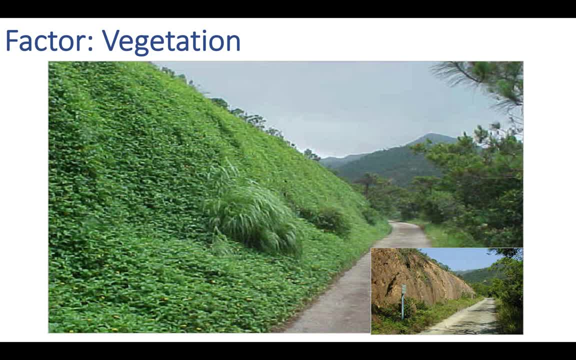 to have a lot of water to stay on the surface of the earth. You need to have a lot of water to stay covered with grass, plants and trees. So the big picture here shows land with a lot of vegetation. The small picture on the bottom right side of the screen is showing the same area that 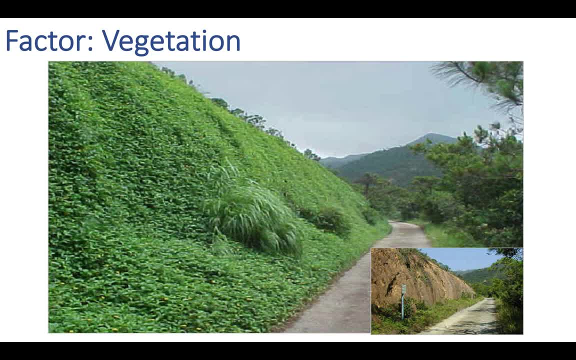 has no more vegetation. When you have vegetation, plants love to soak up water. So when you have vegetation, there's more infiltration. Water is able to go into the ground a lot easier. But on the other hand, when you completely take away the vegetation, there's going to. 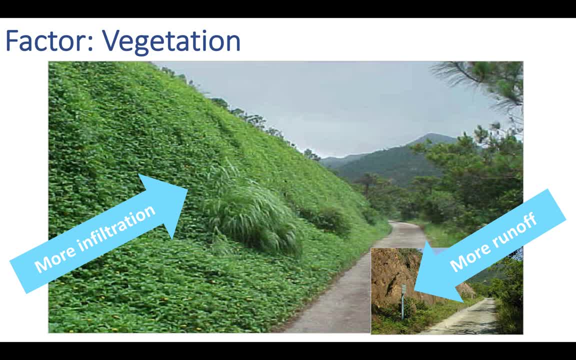 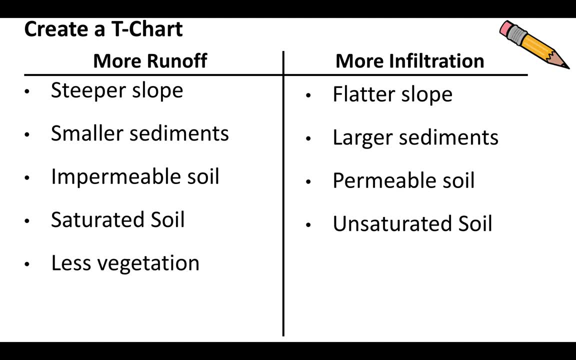 be more runoff because there's less plants to soak up that water, So that water is going to be more likely to stay on the surface. So the last thing you're going to add to those T charts- more runoff is when you have less vegetation. 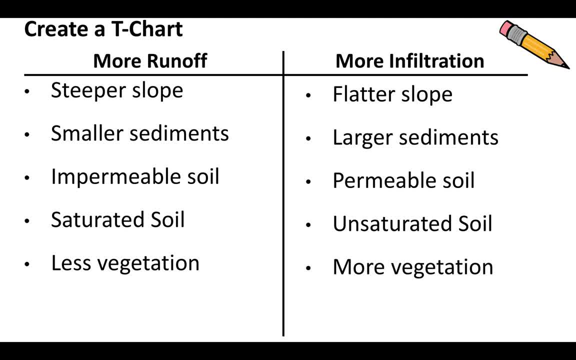 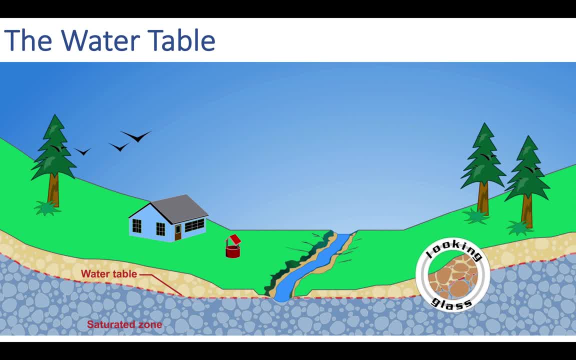 If you want more infiltration, you want to add more vegetation. The last thing I just want to go through today is showing you guys this term called the water table. What you might not realize is beneath the surface that we walk on is a level of water.